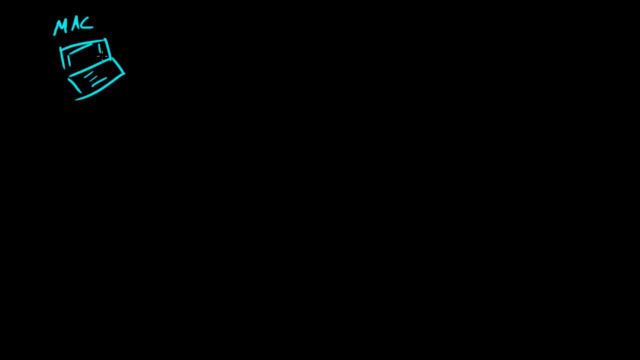 Wow, this is a pretty terrible looking macbook, but oh well, So this is your mac over here and we'll say that you want to, you know, view a website or something. So web server is going to look something like this. So, again, unlike the last example where we had a guy talking to a girl trying to get his number, now we have a mac talking to a web server trying to get a website. It's kind of like the dating, for example. 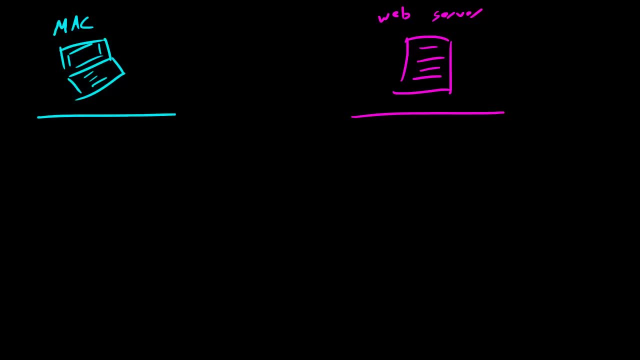 I don't even know why I said that it's pretty stupid. But now let's go ahead and look at a conversation between two computers trying to get a website. So this is basically what happens whenever you request a website. If you're on your mac, the first thing it does is it asks the web server: can I connect to you? So this is the first kind of exchange and what the web server does is it asks the web server: can I connect to you? 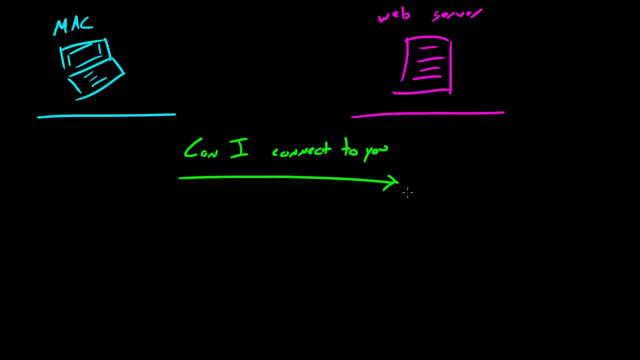 So this is the first kind of exchange, and what the web server says is: if it has permission, then it says yes. For example, if it's a web server, if it's a personal home server, it's going to, of course, say no, But since this is a web server, we'll say it's. I don't know my web server for the new Bostonorg- Best website ever, by the way- The web server is going to go: yes, you have my permission. 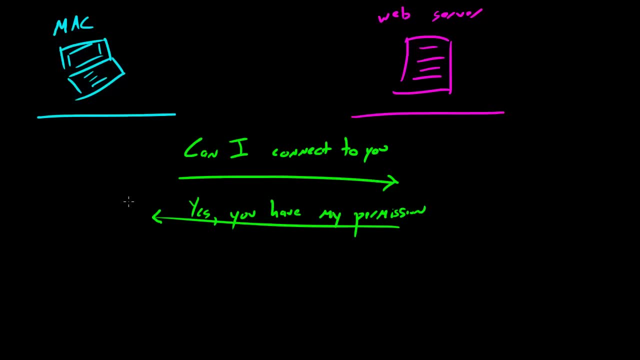 Now the Mac now knows that it now has the authority to connect. So now what it's going to do is it's going to go- yes, you have my permission, gonna request the file, which is, of course, the web file, so we can view the website. so it's gonna send a request that looks like this: get and we'll talk. 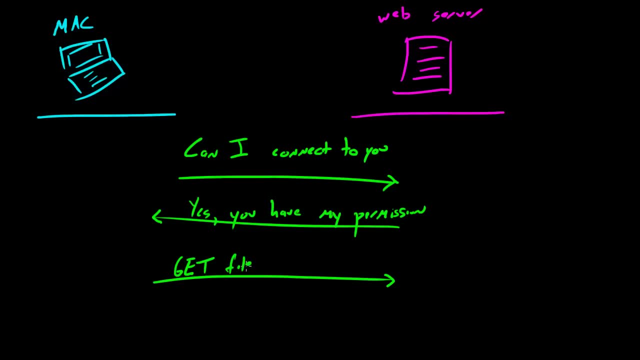 about why I wrote: get in a little bit file, and the file is just gonna be, you know, the new Boston dot org slash index or like tutorials, dot PHP or something like that. so this is basically the file that it's asking for and in return, of course, the web server sends the file to the Mac and, of course, the Mac 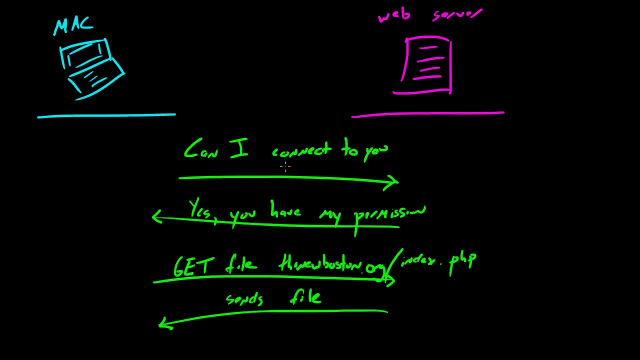 interprets it, views it as a website. everyone is freaking happy. so let's go ahead and take a step back and learn why this exchange was successful. well, first of all, this works because both of the computers- the Mac and the web server- they knew the rules. they followed the same protocol. 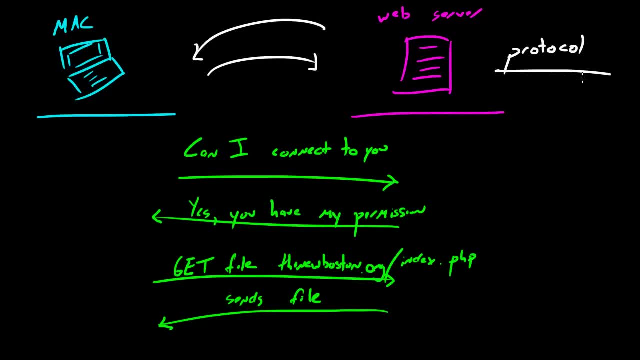 or the same set of rules. now in computer networking, both the computers, this one and this one, they must follow the same protocol, or else you can't have a successful communication, you can't have computer networking at all. now, of course it was a lot easier to understand. whenever we're talking about human 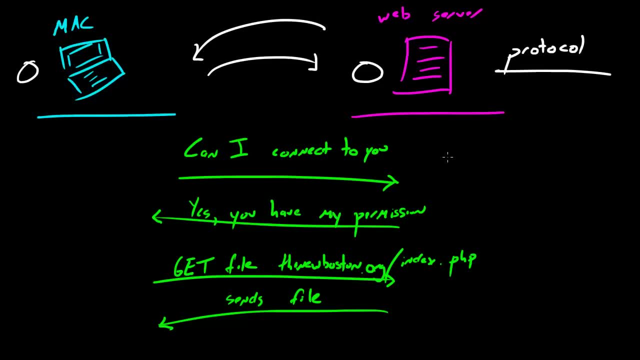 beings, the different rules, but the protocol, pretty much the protocol in computer networking, is the format, and we'll look at this later. it's different for every protocol, the format in the order of messages. those are two big ones. so of course, if this Mac, you know, asked for a file before it even had permission, this exchange 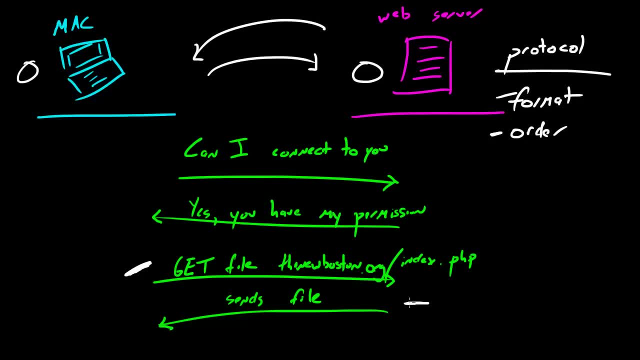 wouldn't work. or, you know, if the web server was trying to send a file in this Mac over here, it didn't even ask for a file yet- then of course, you know, things would get really messy and computer networking would not be possible. if you know, every web server in the world would not be able to send a file to a computer. 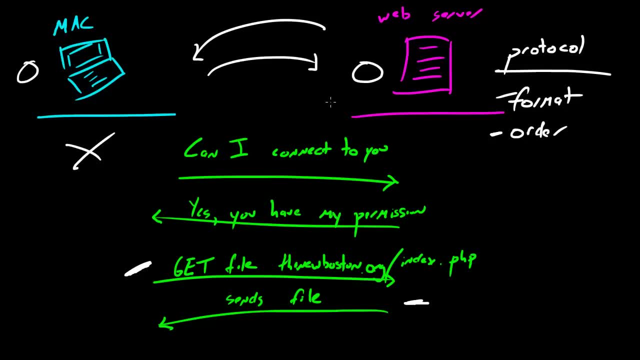 with just sending random files out. probably, you know, the internet wouldn't be as successful as it is today. so that's the basics of what a protocol is in computer networking and also, you know, a human being protocol, basically a set of rules that both computers must follow in order to have a successful 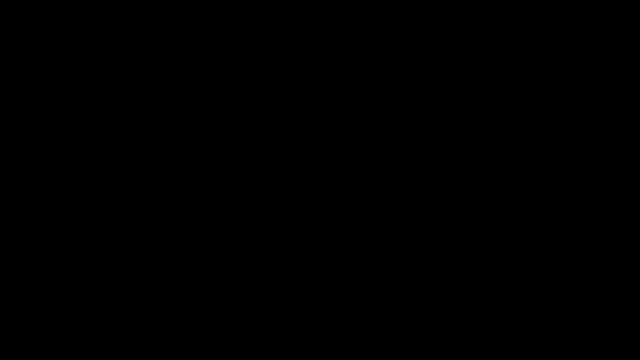 communication. now let me go ahead and show you guys something else real quick. that's pretty cool and you guys may have seen this before: this protocol right here. well, I'll talk about the different types of protocol in a second, but whenever you look at a URL, you're gonna 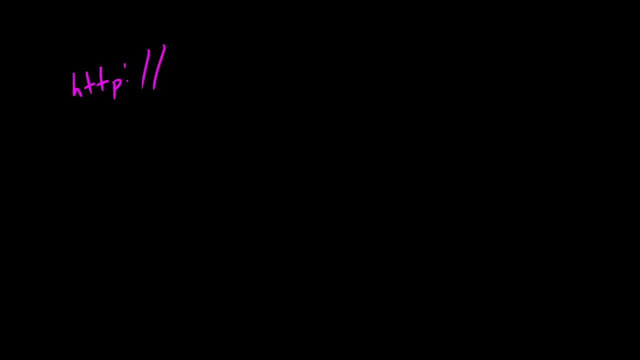 see something like HTTP and let me write these in different colors: wwwthenew probably gonna run out of room, bostonorg and what's- another color I didn't use- and we'll just write like slash index dot PHP. so now, if you guys, you know, used to type in URLs and you guys didn't really know. 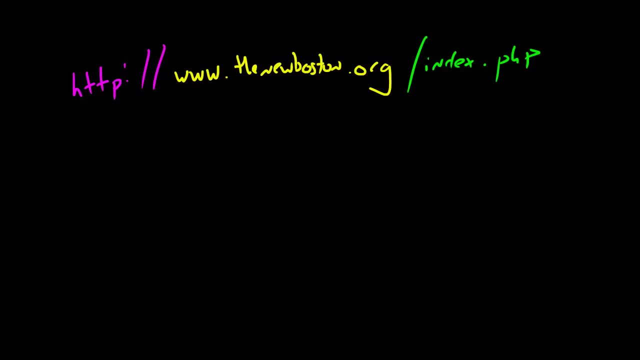 what you're typing in now. you have enough knowledge of computer networking to understand everything. the first part right here: this HTTP, this is the protocol, hopefully a protocol protocol. wow, I cannot spell. so this is actually a hyper text transfer protocol and again, like I said, there are a lot of different. 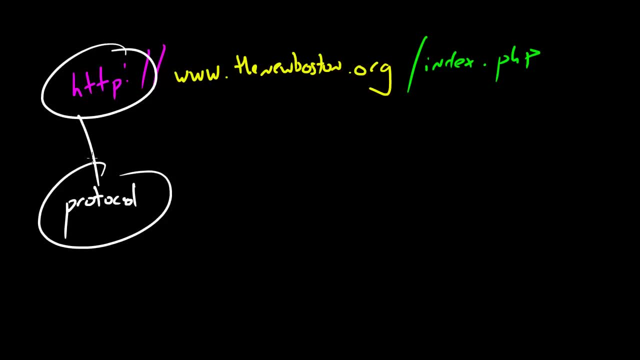 protocols or sets of rules in computer networking. whenever you want to request the website you know from the world wide web or the internet, this is the protocol over or the rules that your computer has to use this right here: wwwthenewbostonorg. this is actually the name of your server. server name. 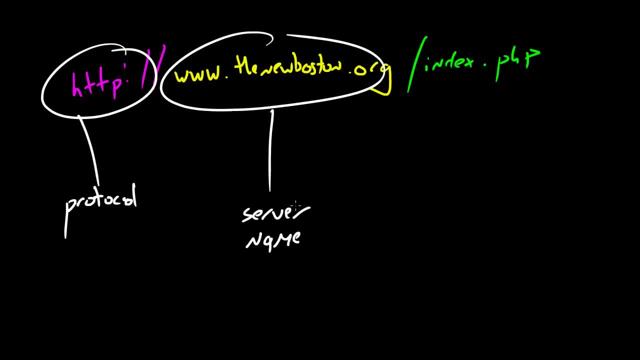 because, remember, a server is just a special computer. so, of course, whenever you want to ask for a file, which is this part right here, a file from a computer that somewhere out in the world, you need to know again the address of the computer, because you just don't want to ask random computer. 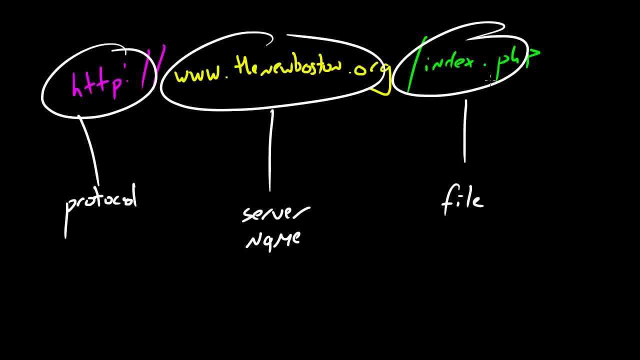 for files only a specific computer. so this, of course, is the file. so again, whenever you want, say, to look at a website on my webpage- yeah, that's what- or a webpage on my website. rather, we're going to do, is you're going to say, okay, I want to ask this server for this file and I'm going to use this protocol, which? 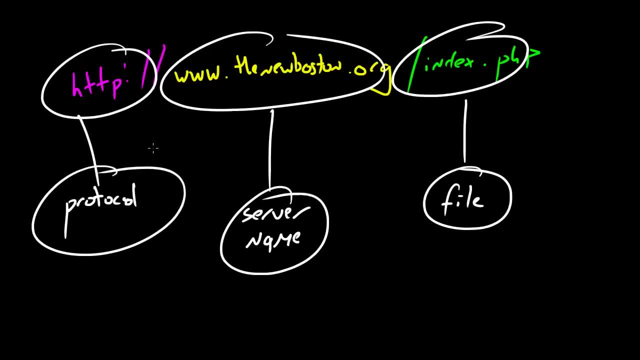 is basically the set of rules that my server knows it's already set up. whenever you request a website, this is the rules that you must follow. So again, hopefully you guys understand a little bit about protocols and, if you don't, and this goes for the rest of my tutorials- 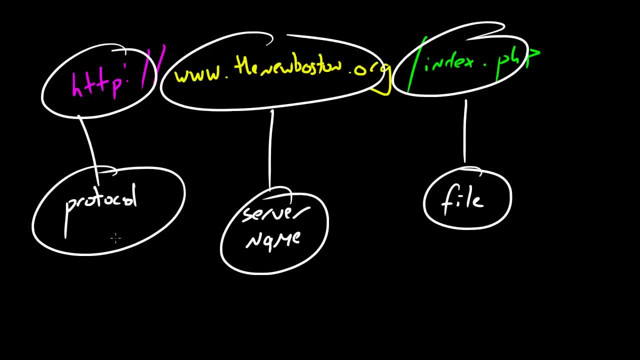 if you guys have any questions, then just go ahead and ask me on Facebook or Google plus or even Twitter, or the best place is probably my forum on my website, Because if I don't answer you, there are thousands of other people willing to. so anyways, thank you guys for watching.